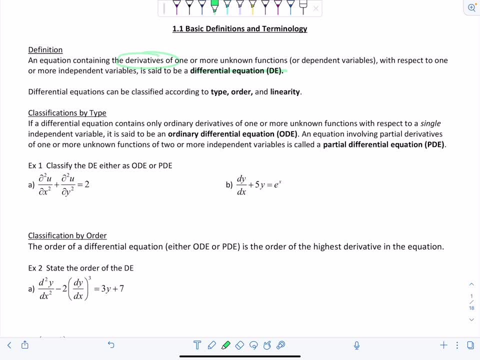 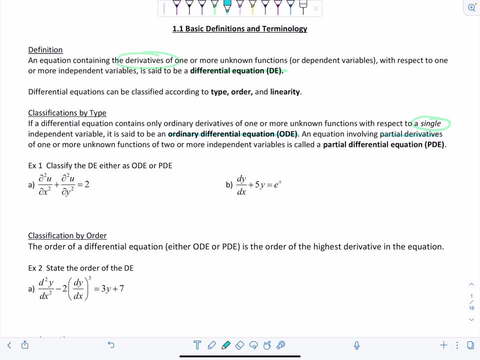 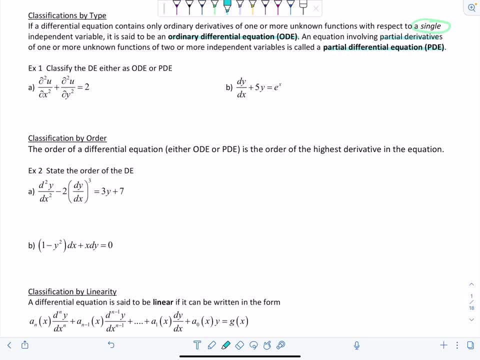 So example one: classify the DE, the differential equation, either as ODE- ordinary differential equation or PDE- partial differential equation. I mean, what can I say? We just love abbreviating in math, right? We're not all about writing down long words all day. 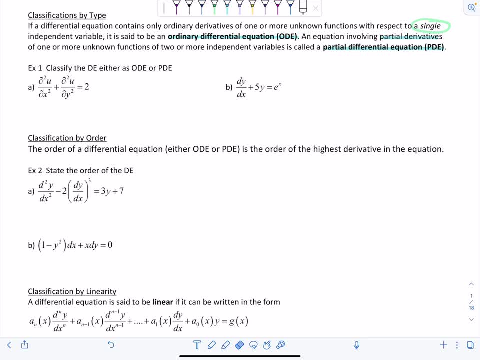 So example A- maybe it's staring you right in the face- We can tell that there's partial derivatives going on right. Remember del. when we switch our notation, it means that we're taking a partial derivative. In fact, here this equation is the second partial derivative of U, with respect. 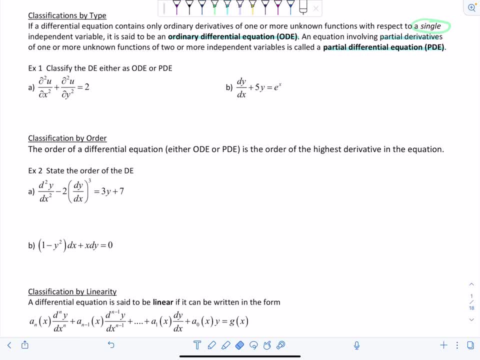 to X, plus the second partial derivative of U with respect to Y, and this equals two. So as soon as you notice- right, we have del's instead of D, then you know we're taking partial derivatives. So that's going to make this a PDE partial differential equation. 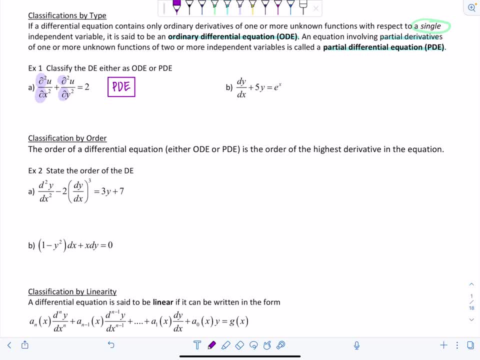 All right, and let's identify what the independent and dependent variables are. So notice: the dependent variable is U, and U is a function of what we can tell so far: X and Y. So U is a function of two or possibly more. 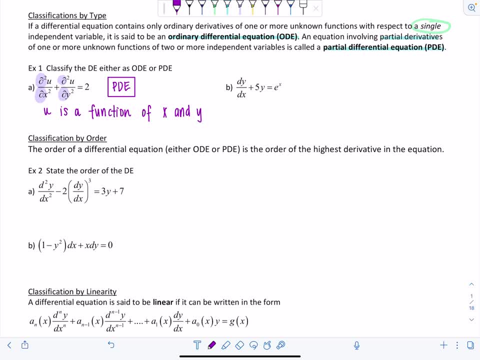 independent variables and notice this equation includes partial derivatives. PDE, All right. example B: notice we have DYDX plus 5Y equals E to the X DYDX. that's an ordinary derivative right. We're not taking a partial derivative. And Y is a function of. 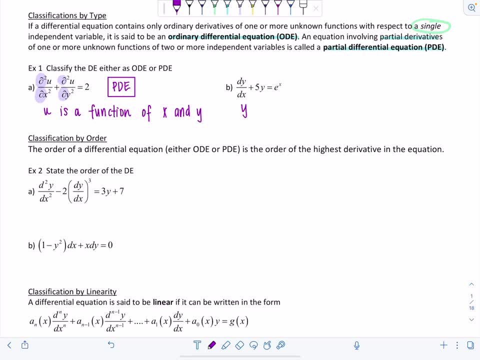 a single variable, just X. So Y is a function of just X and this is an ODE, ordinary differential equation. All right, so that's the difference, or the two categories, when we talk about type, either ODE or PDE. Now let's talk about the next classification, which is order. Now the order of a. 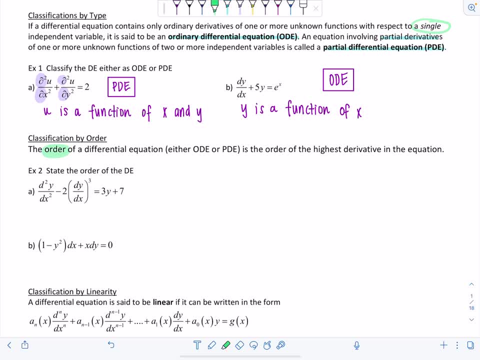 differential equation, and this can refer to both ODEs or PDEs. okay, We can both say what their order is. That's the order of the highest derivative in the equation. All right, so why don't we just go back to? 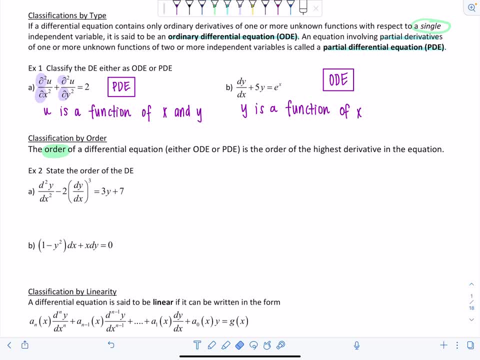 example one and figure out what the order is for each of those differential equations. Look at what the highest derivative is in the equation. okay, So for example, A notice we have- we have second partials, So the order of that equation would be two because we have a second derivative in there. 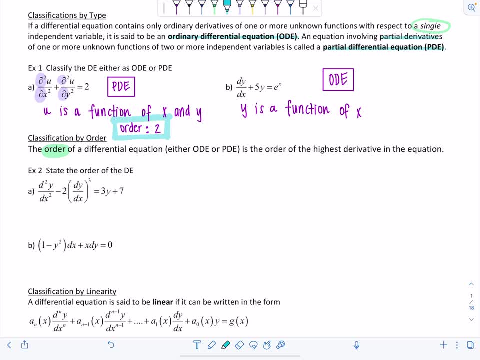 That's the highest one that I see. So order is two. What about example B? I just see a first derivative right, DYDX. So that means the order is one, All right. so notice: this classification applies to both PDEs and ODEs. 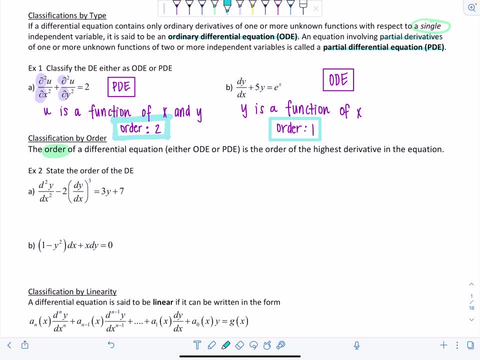 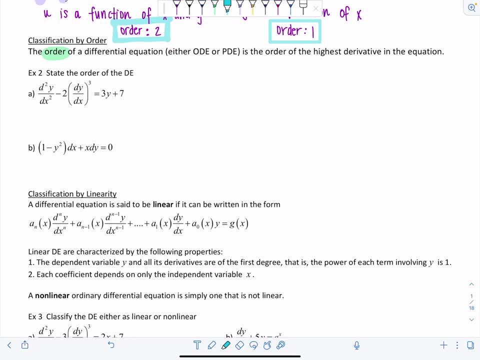 You can identify their order. All right, let's look at some more examples and figure out their order. For example, A notice: we have D squared, Y over DX squared, So that's going to be our second derivative of Y with respect to X. 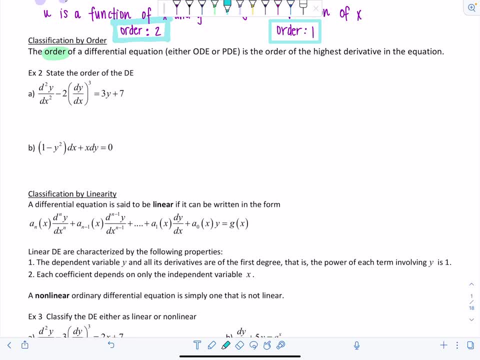 minus two times DYDX cubed equals three Y plus seven. All right, so, first of all, is this: is this an ordinary differential equation or partial differential equation, ODE or PDE? I know they didn't ask, but we're just being over achievers. Yes, 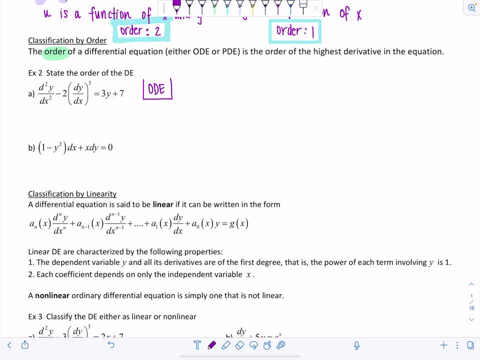 It's an ordinary differential equation, right? There's no partial derivatives here. Now let's figure out the order. What is the highest derivative that you see in the equation? Now, don't be fooled, This is not a third derivative. This just means you take DYDX. 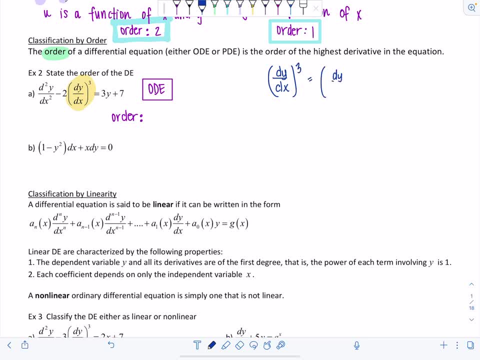 and you cube it, So you have dy dx times dy, dx times dy dx. How is that different than the third derivative? Well, the third derivative we would write this way if we were using Leibniz notation, So you would have first, you'd start with the derivative dy dx. 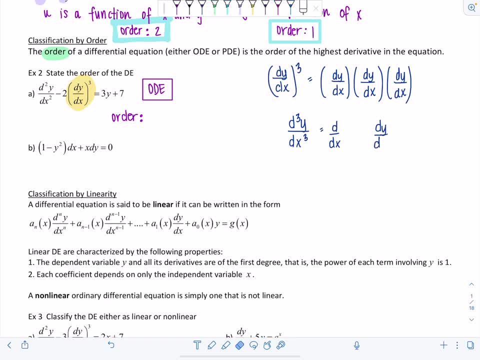 Oh, what am I writing, dy dx, excuse me. And then you would differentiate again with respect to x, and again right, And that would be your third derivative. Okay, note the difference. These are different. Okay, so don't get confused. 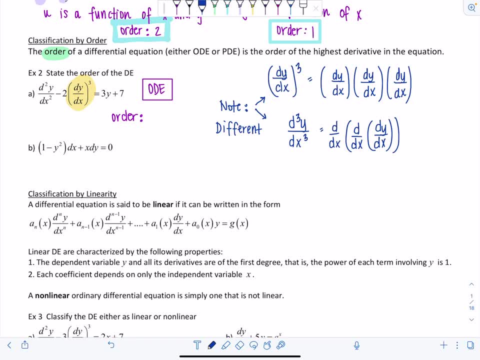 That's not a third derivative in equation for A. That means: what's the order of that differential equation? Yes, it's just two, because the highest derivative in the equation is that second derivative. Okay, good, Let's look at example B. 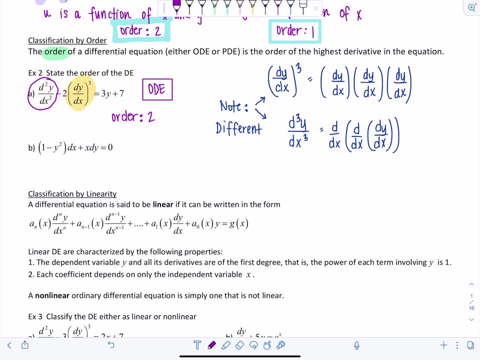 First of all, is that an ODE or a PDE? You might be thinking. this doesn't even look like a differential equation to me. It just needs a smidge of rearranging. I agree, Let's divide everybody by dx, Okay, and then now it should look a little more familiar. 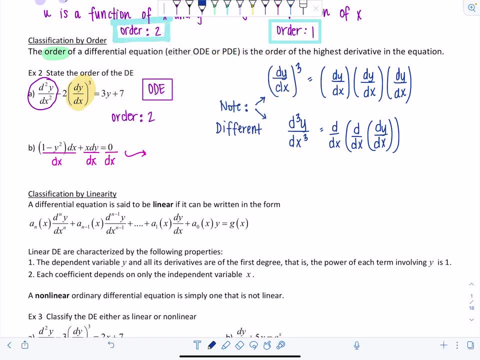 So we're going to have just 1 minus y, squared plus x times dy dx, and that'll still equal zero. Okay, now let's start classifying. So no partial derivatives, just ordinary derivatives. That makes this an ODE. And then, what is the highest derivative that you see? 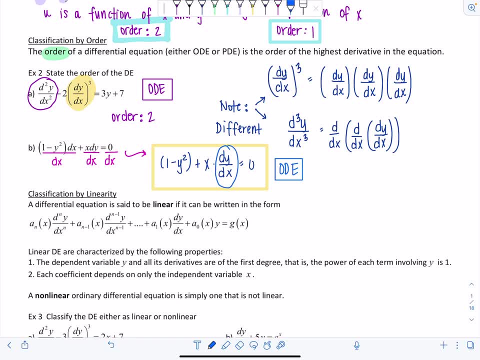 Well, the only derivative I see is dy, dx. So that's going to make this order 1.. All right, very nice. So that's how we classify the order. Last classification deals with linearity that we're going to talk about today. 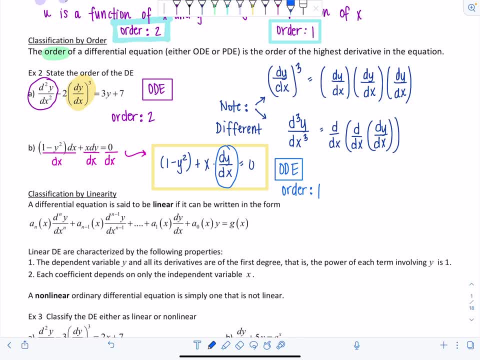 A differential equation is said to be linear if it can be written in the following form: And this might look a little wild, but we're going to break it down right now so you can understand what exactly is going on. So notice: you have a sub n of x. 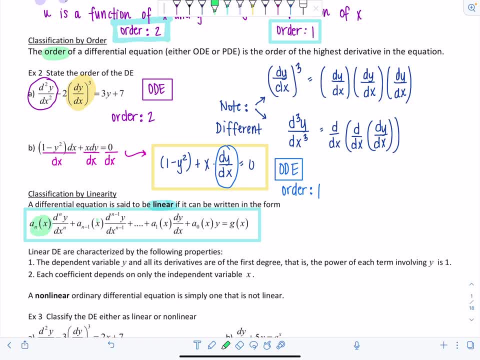 a sub n minus 1 of x, And these are all basically functions of x that appear in a linear differential equation And they are attached to or multiplied by notice here- derivatives of y with respect to x. All of these derivatives are of the first degree. 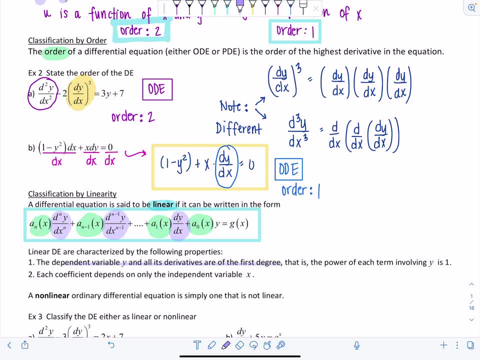 So that means we wouldn't see derivatives being squared. We could see higher order derivatives. that's totally fine, but the derivatives themselves are not raised to any powers other than 1.. So the power of each term involving y is 1. And the power of each term involving y is 1.. 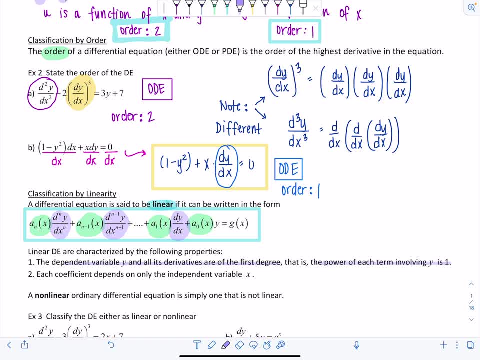 The second criteria for a linear differential equation is that the coefficients- all of those a sub n of x's that I highlighted in green- each coefficient depends only on the independent variable x, So it should not be a function of y. You shouldn't see any y's floating around out. 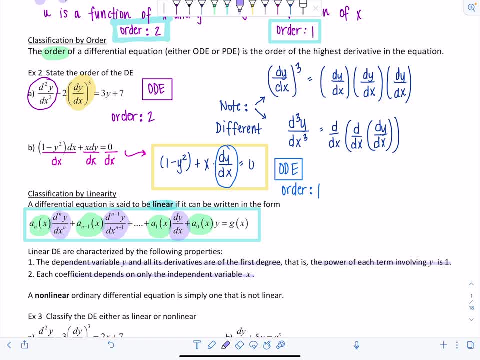 there You can have one plain old y. notice right here that you didn't take the derivative of. That's fine. Remember though the exponent on it has to be a one. but you can't have a function of y, Just y, derivatives of y with respect to x, and then functions of x are allowed. 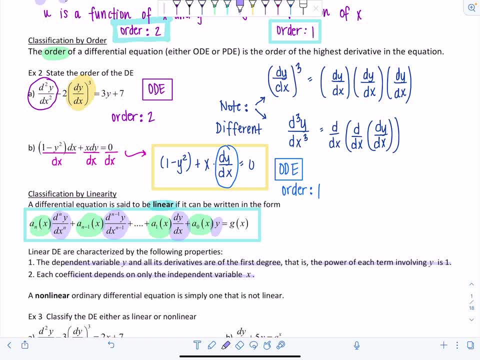 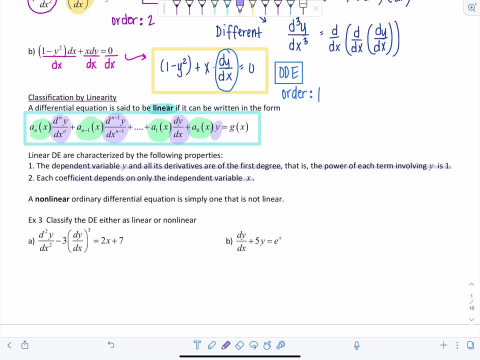 Okay, It might take a few examples for you to get this straight, but don't worry, I got you. Here we go, And if it's not linear, you just say nonlinear. Okay, This applies for all of the examples that we did so far, so we can revisit them too. 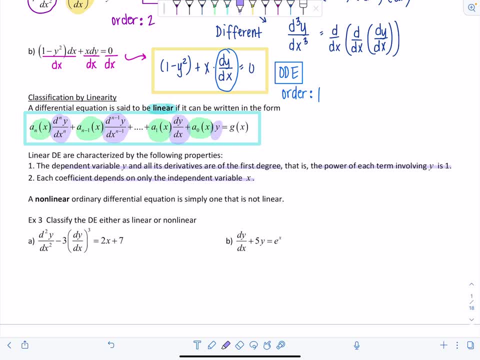 So classify the differential equation as either linear or nonlinear. So first term is a second derivative of y with respect to x. that's fine minus three, and then I have dy dx cubed. Oh, that's a problem right there. 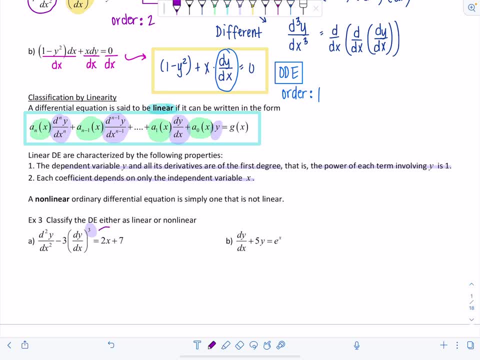 because the exponent on the first derivative is a three. So that makes this equation, right here, nonlinear. If the exponent was a one, then it would be linear. we would be fine. Okay, Good, Let's look at example B, which actually was example B in problem one. We have dy dx plus five y. 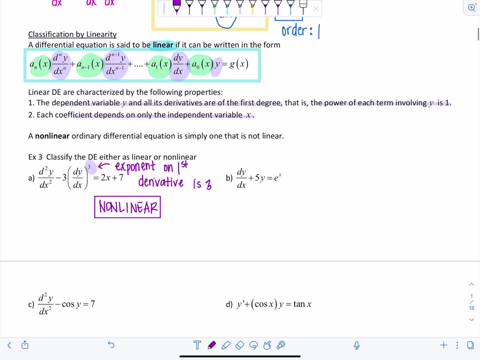 equals e to the x. All right, Now notice, here we have the first derivative, but it's raised to the first power. There's no extra exponent on it, right? So this is raised to the first power. We also have y raised to the first power over here. five is basically that a sub n of x. 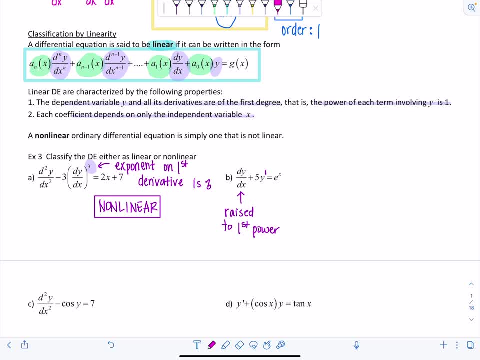 it's a function of x, it's a constant, and then this equals e to the x. that's fine. g of x is a function of x, So it looks like it satisfies all the criteria that we have for a linear differential equation. So that is how we're going to classify this guy. This is linear. 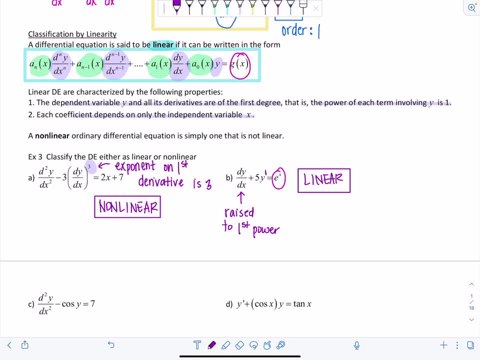 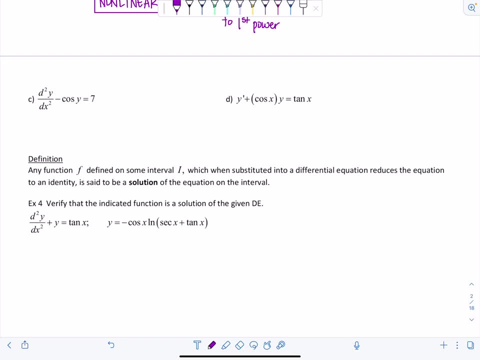 Fabulous. Okay, a couple more. We have second derivative of y with respect to x. That's fine, That's a second derivative, but it's just being raised to the first power, right? This is all to the first, so that's okay. Minus cosine of y equals 7.. Now this: 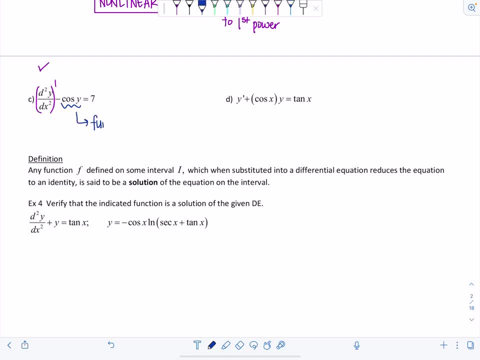 is going to be a problem for us. This is a function of y And, remember, we can only have functions of x appearing in linear differential equations. You can have y or its derivatives, but you can't have functions of y, So that makes this nonlinear. 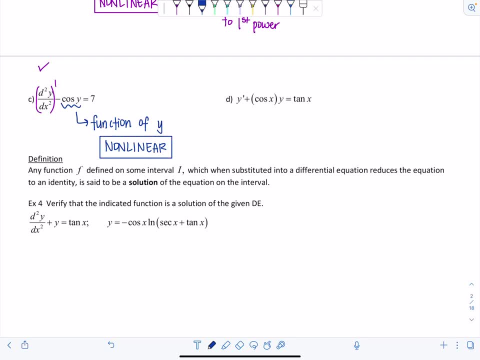 And last example: we have y prime plus cosine x times y equals tangent x. Let's replace y prime with our other notation, So we'll write dy dx plus cosine x times y equals tangent of x. So let's see dy dx. fine, That's the first derivative. It's just raised to the first power I have, y. 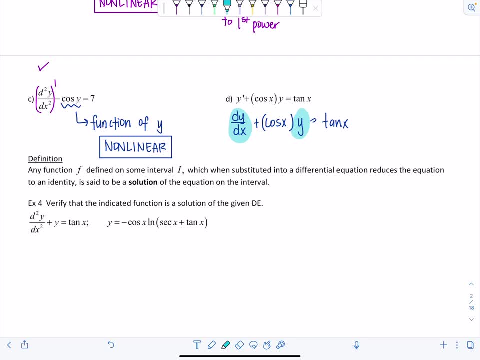 That's raised to the first power. It's not squared, It's just raised to the first power. It's not squared or cubed or anything like that. Cosine x, that's the a sub n, Remember, that's the coefficient there And that's a function of x. Okay, no problem On the right. 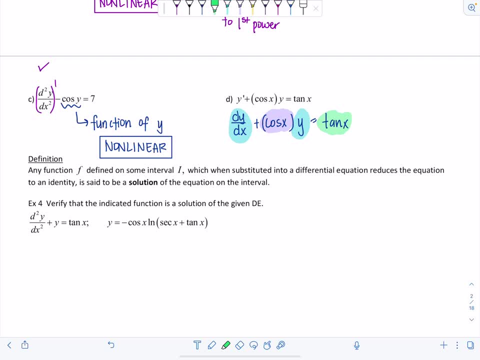 hand side, I've got tangent of x. I think that's like the g of x in the definition for the form. So it looks good. It looks like it passes all the criteria. So this is a linear differential equation. Now why do we classify these? 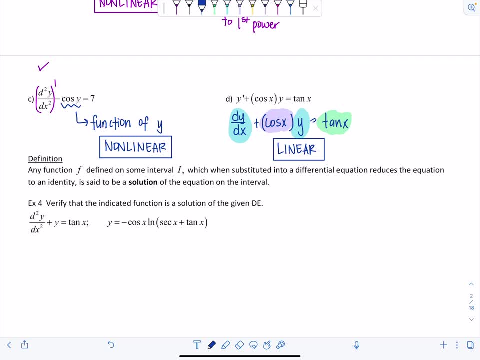 Why is it a linear differential equation? Because it's a linear differential equation. Is it a big deal? Because, as we learn throughout this course how to solve the differential equations, choosing the appropriate technique begins by first correctly identifying what sort of differential equation you're dealing with. All right, And of course we're going to add. 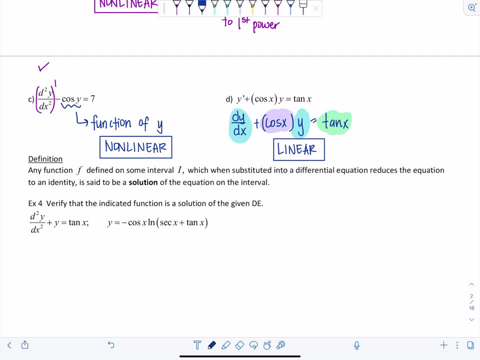 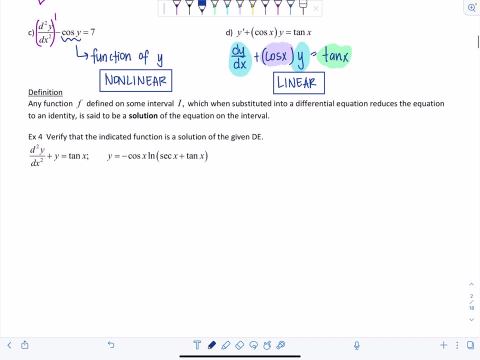 to these definitions and get more specific and learn about more types. But this is just laying the foundation. Now, another definition we have is that any function f defined on some interval- i So basically think, like where it's well defined, the values of i fall within its domain. 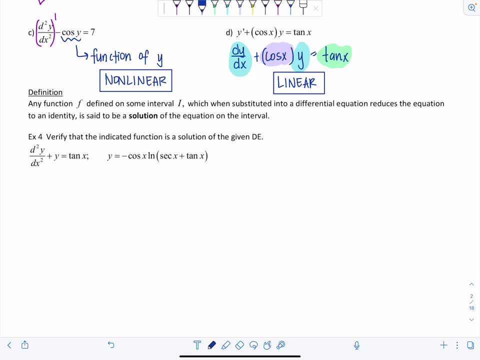 which, when substituted into a differential equation, reduces the equation to an identity, is said to be a solution of the equation on the interval. So when you solve differential equations, you're finding functions or equations that, when you take their derivatives, will satisfy the differential equation when you substitute them. So when you take their derivatives, 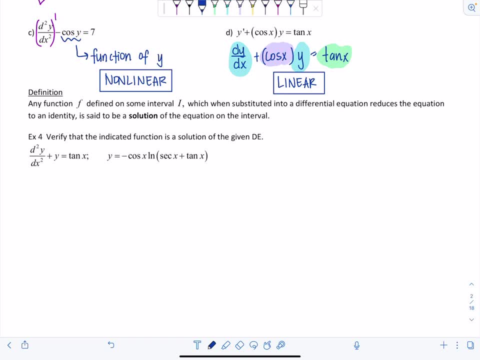 you substitute them back in. We'll learn how to do that later. That's what this whole course is about. But right now, in the next example, all we're going to do is verify that the indicated function is a solution of the given differential equation. So here's our 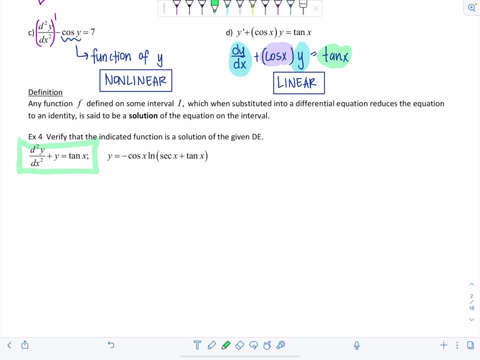 differential equation. We've got second derivative of y with respect to x plus y equals tangent x. That's the differential equation. Right here they're giving us the solution of the solution. They're saying: y equals negative cosine of x, ln of secant x plus tan x. That will. 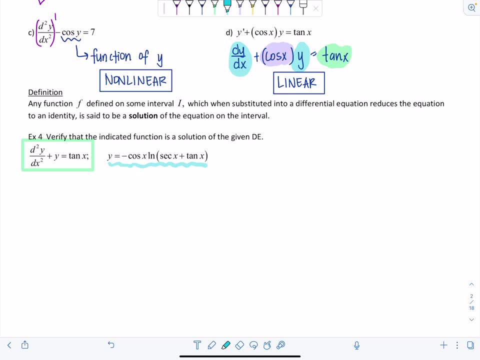 satisfy the differential equation. So how do I verify it? Well notice, my differential equation involves a second derivative. So I'm going to go ahead and differentiate this equation. I'm going to differentiate y with respect to x twice. substitute it in there, where the second derivative 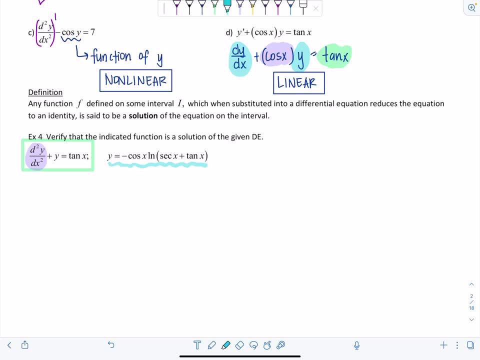 is, Then I'm going to go ahead, substitute in the original derivative. So I'm going to go ahead and substitute in the original function y and verify that it gives me back tangent of x. That's how I know it's a solution to the differential equation. Now, this derivative will not be for the faint of. 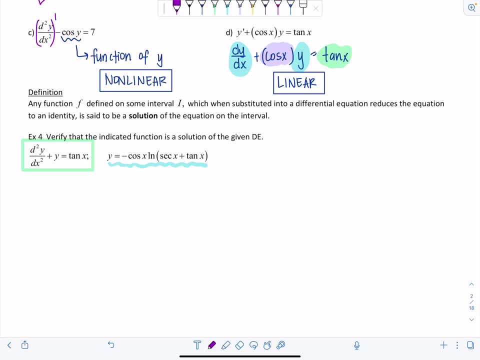 heart. So let's focus so we don't mess up. okay, Here we go. So dy dx notice right off the bat, it's product, real time people. Yes, do you see that? So we've got negative cosine x. 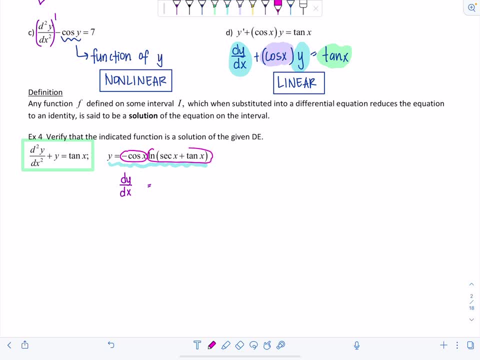 and ln of secant x plus tan x. Okay, so for the product rule, remember each of the functions takes turns having their derivative taken. That's how I like to think of it. So, derivative of negative cosine x, dot sine x. 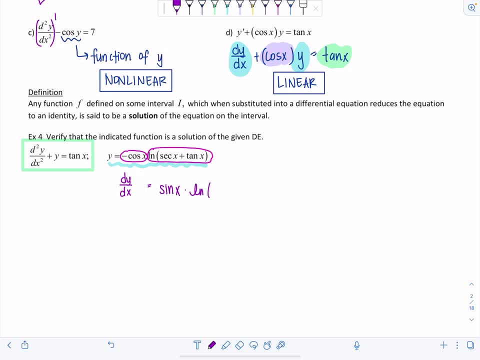 And then I'm going to leave the other function alone. So leave alone good old ln of secant x plus tan x. Plus, now we're going to leave alone the negative cosine x and then take the derivative of ln of secant x plus tan x. So remember: derivative of ln of secant x plus tan x. 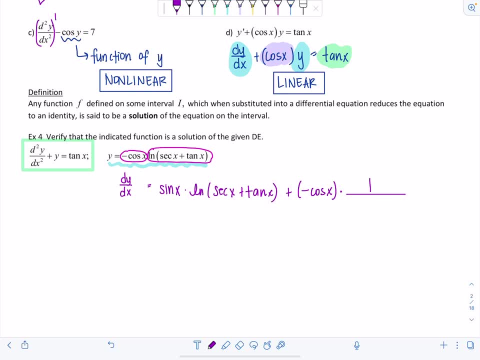 And then by the chain rule, I have to multiply by the derivative of the argument or what's inside those parentheses. So the derivative of secant x- we know it right. Of course we didn't forget any of our good calculus. one material, So that's going to be secant x plus tan x, And then I'm going to 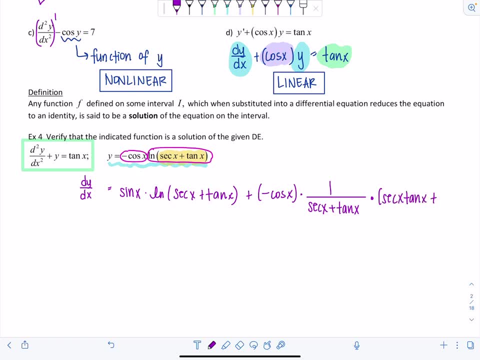 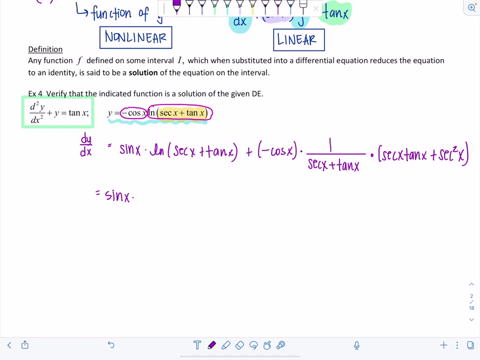 leave the derivative of tan x, which is secant squared x. Okay, right now this is looking like a hot mess, But look, we can clean it up just a bit before we continue, because I need another derivative, right, My goodness. Okay. so we have here sine of x times natural log of secant x plus. 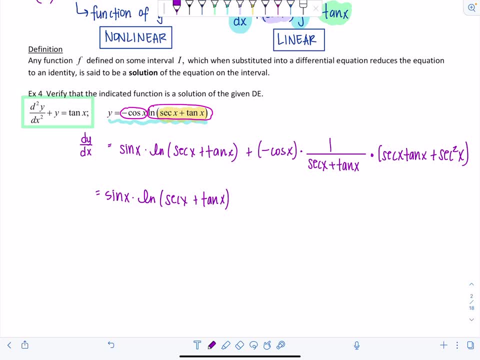 tan x And then minus cosine x. I'm just going to put that over here. So I'm going to put that over: secant x plus tan x, And maybe you noticed already I can factor out a secant x from this expression here. So now I'm going to have secant x times tan x plus secant x. Woohoo, That's good. 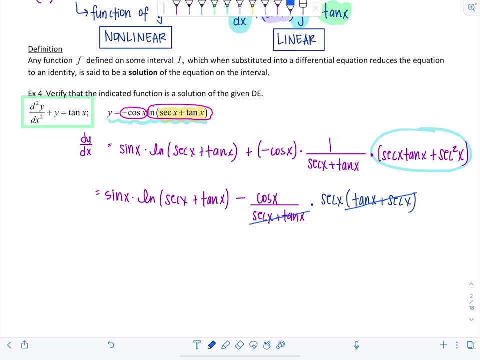 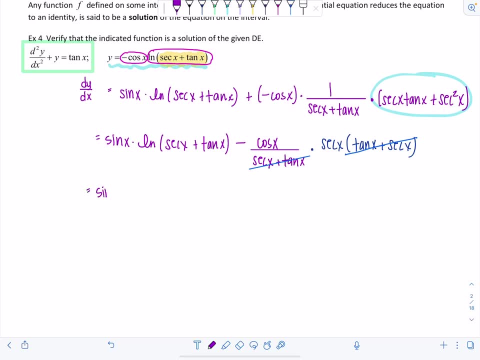 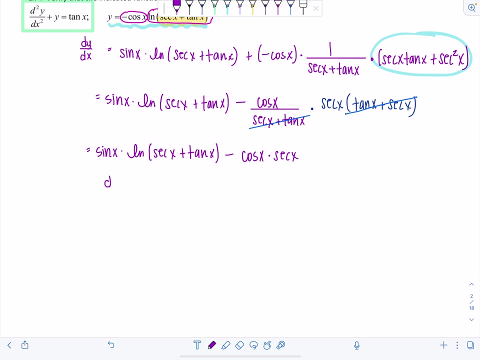 because now I can cancel out secant x plus tan x, And let's see what else Things are shaping up nicely Here. we've got sine x times ln, secant x plus tan x minus. all that's left over now is cosine x times secant x. Oh, but wait, secant x is 1 over cosine x, So I can write my final result: dy dx. 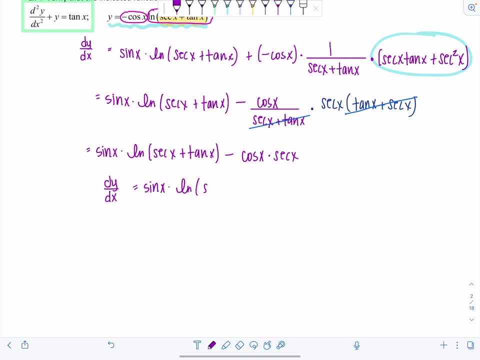 as sine of x times ln, of secant x plus tan x minus 1.. Woo, Okay, Now from here we can differentiate one more time, and then we'll be ready to substitute everything in and verify that this was the solution to our differential. 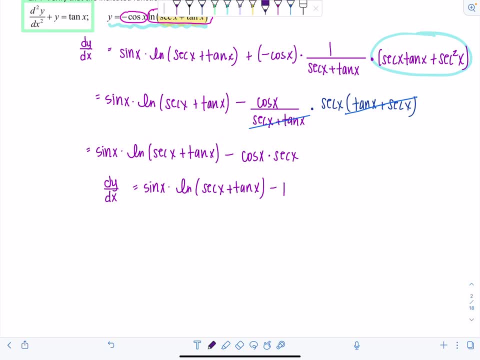 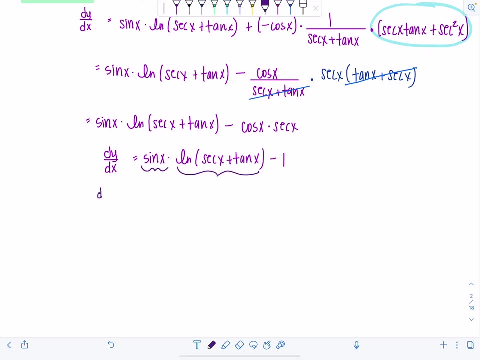 equation. So second derivative time, here we go. Yes, we need to use product rule again. Do you see that, Mm-hmm? Okay. So second derivative: Okay, Derivative of sine x is cosine x. Leave alone ln of secant x plus tan x, Plus, leave sine of x alone. 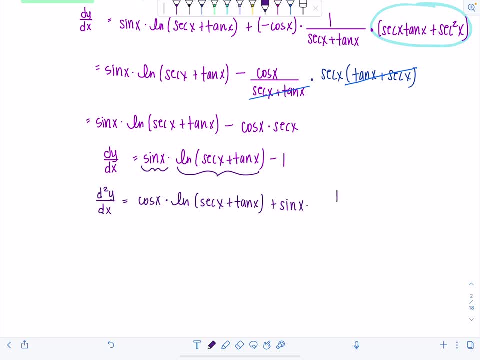 Derivative of ln of secant x plus tan x. we just did it right: 1 over secant x plus tan x times by the chain rule: secant x- tan x plus secant squared x- Même. Okay, we're going to do the same thing as before. 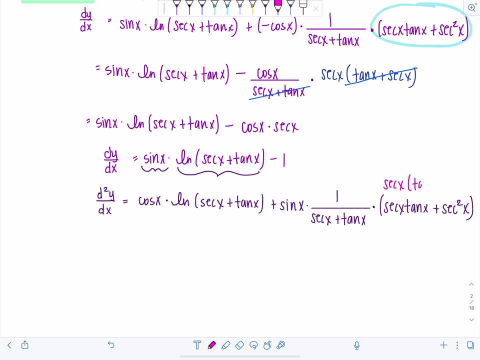 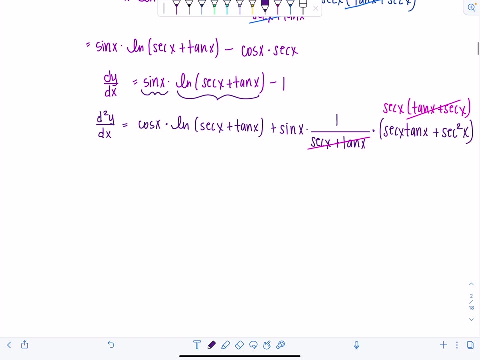 To clean up, remember: you can take out a secant x here. then you're left with tan x plus secant x, right, And so you can cancel out the secant x plus tan x, and now we're left with cosine x. 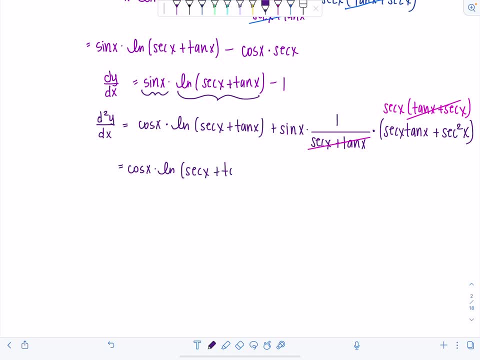 times ln of secant x plus tan x plus. Now, What survived in that term? over there We've got a sine x and a secant x. Okay, can I clean that up a bit more, Of course. So secant x is 1 over cosine x. So sine x times secant x is going to be: 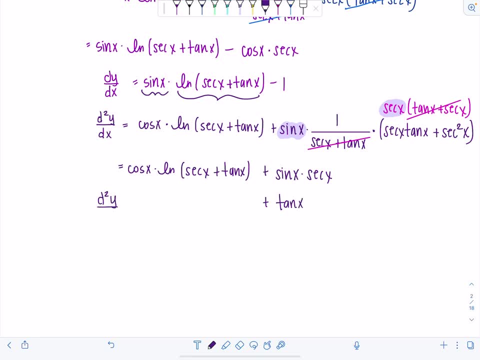 tan x. So here's our totally cleaned up. oops, I forgot that 2 there for the second derivative, So sorry. And this is now what we're going to substitute back into the differential equation. All right, what was the differential equation? Let me remind you. Okay, let's box this. 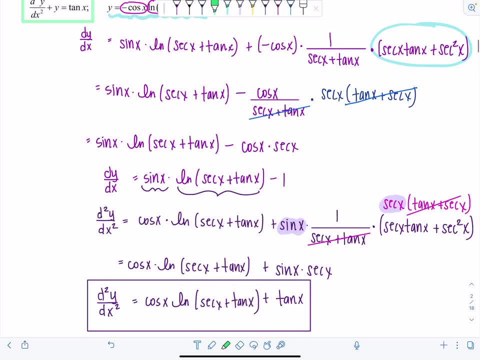 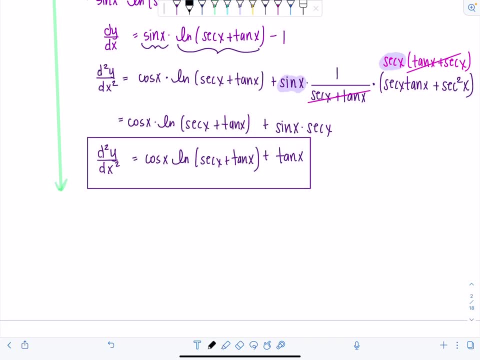 The differential equation's all the way up here. I'll just rewrite it. So the original one, because we have our second derivative with respect to x plus y equals tangent of x. So let's see, here I'm going to replace the second derivative with what we have here. 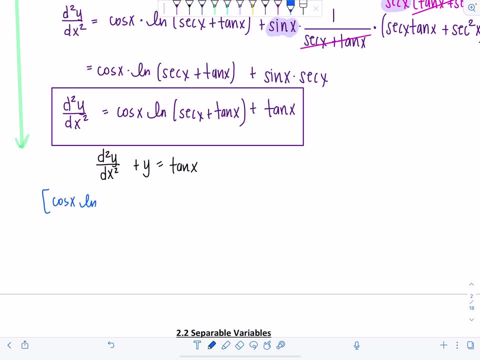 So cosine of x, ln, secant, x plus tan x plus tan x. Okay, that's the second Second derivative. Let me color code for you There: there plus y, y is the original solution that they gave us. So what did we start differentiating in the first? 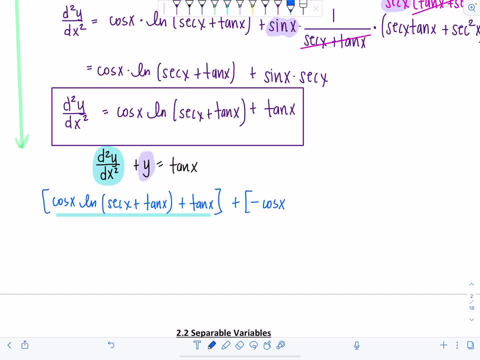 place It was negative cosine x, ln of secant x plus tan x, And I want to know: does that equal tan x? Okay, so, first term, right. there is my second derivative. This is y, the solution that they gave us, and does that equal tan x? 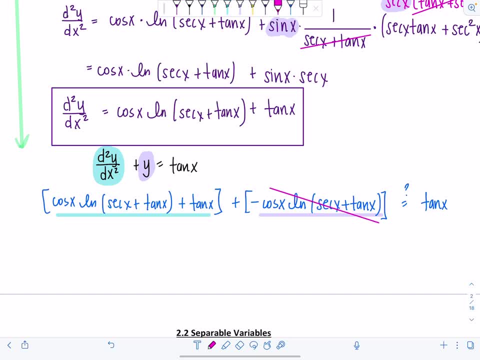 Well notice. Wow, this is just going to cancel out, because I have a positive cosine x, ln secant x, plus tan x and a negative of the same thing. So all that's left over on the left-hand side is tan x, And indeed that equals tan x. 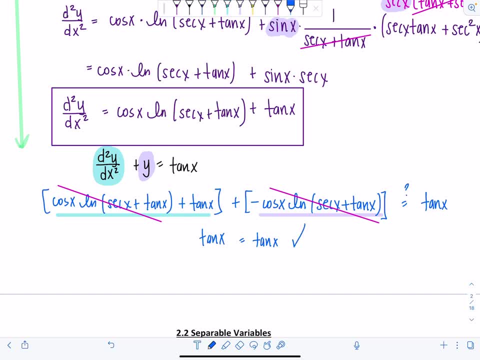 So let's do that check mark with more emphasis. Boom, Yes, Okay. so what does that mean? That y is indeed a solution of the differential equation. It's just an ordinary differential equation. Let's let them know. we know, Okay, and that's it. 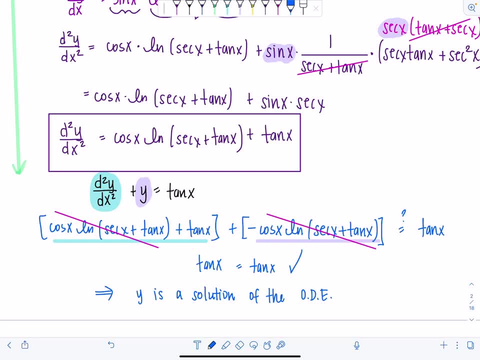 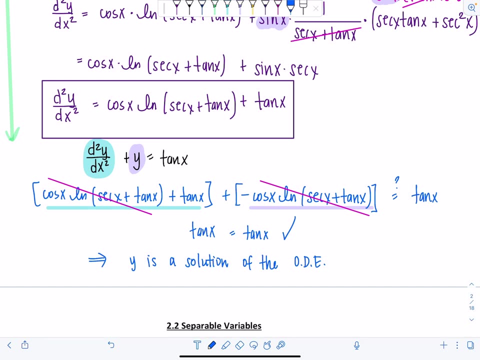 Now, of course, we're not just going to sit around verifying solutions all day. We want to know how to find them ourselves, And that's what we're going to cover over the next several videos. But this is just laying the foundation, And stay tuned. I'm sure you already saw the little sneak peek. separable variables is coming up next. 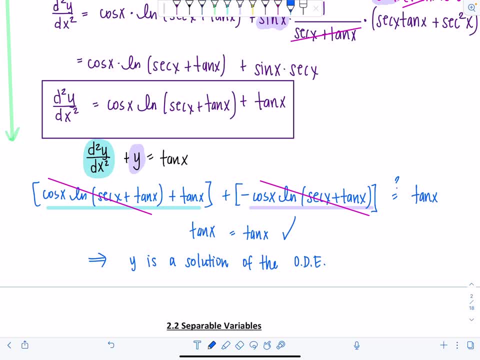 Be sure to give this video a thumbs up. share, subscribe if you haven't already, and stay tuned. We've got more uploads coming your way.